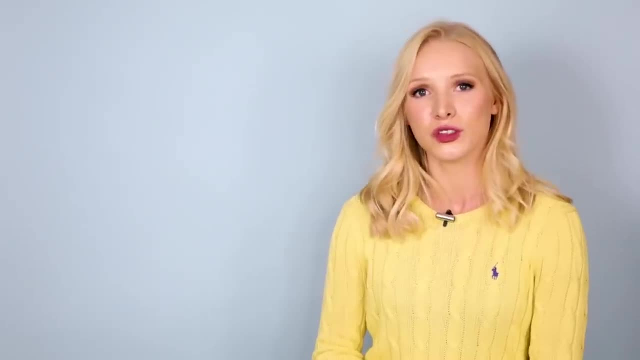 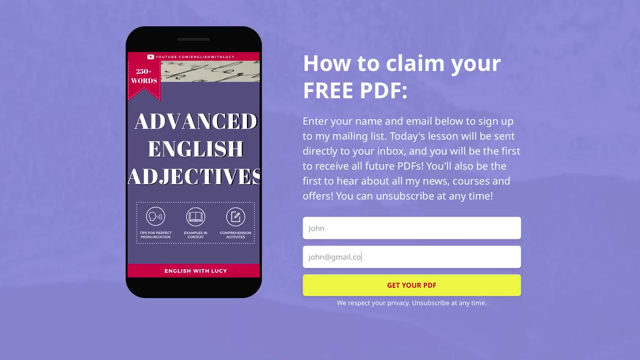 If you would like to download this free PDF, all you've got to do is click on the link in the description box. You enter your name and your email address, You sign up to my mailing list and the PDF will arrive directly in your inbox. 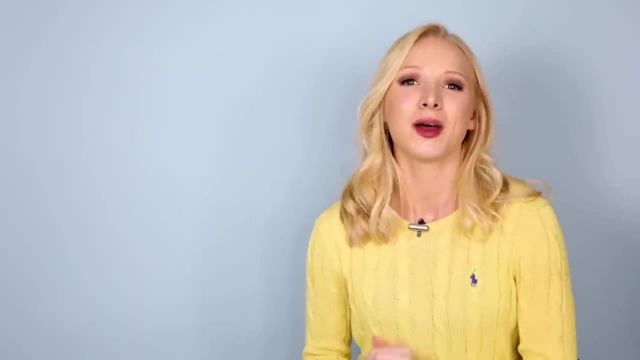 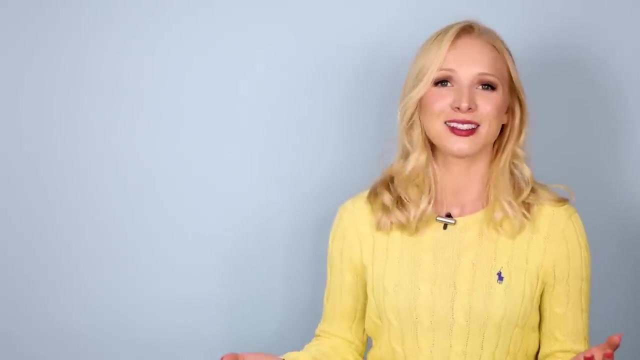 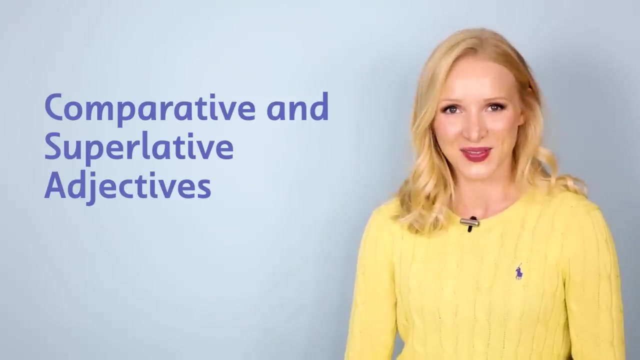 After that you've joined the PDF club, You will automatically receive my free lesson PDFs, along with all of my news, updates and offers. You can unsubscribe at any time. Today we're going to discuss comparative and superlative adjectives. 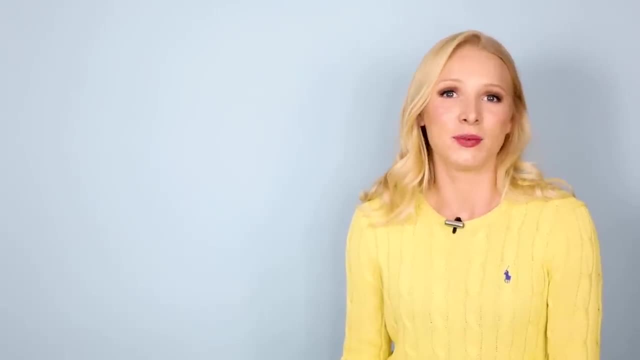 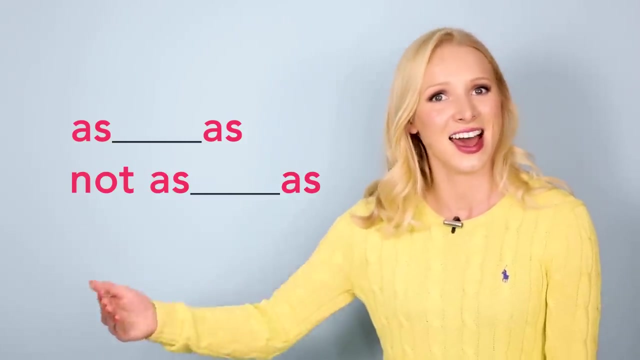 You likely already know that adjectives and adverbs modify nouns and verbs And it's possible to make comparative sentences simply using an adjective or adverb, using the as, as or not as As as pattern. For example, she is as pretty as her mother. 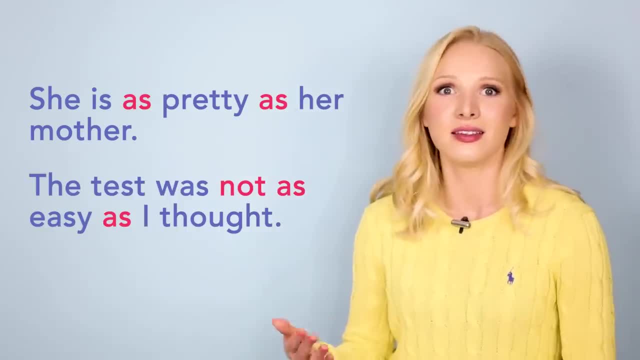 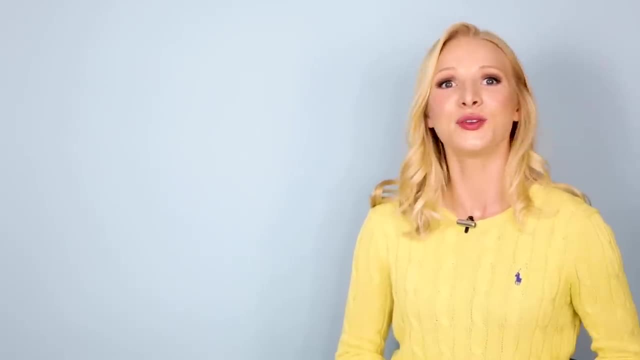 or the test was not as easy as I thought, But today's lesson will focus on making comparisons using comparative and superlative adjectives. Comparatives and superlatives for short A. comparative is used to compare two nouns, Words like faster, slower. 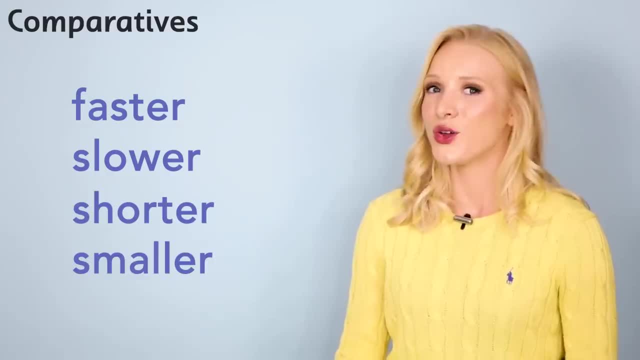 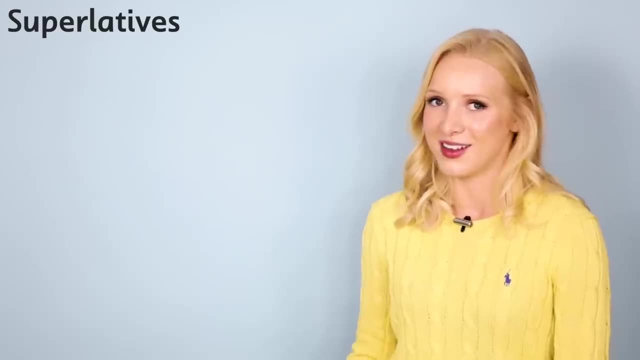 shorter, smaller. Notice that comparatives often end in E-R a, but not always A superlative is used to compare three or more objects that are at the upper and lower limits of quality. Words like the fastest, the slowest. 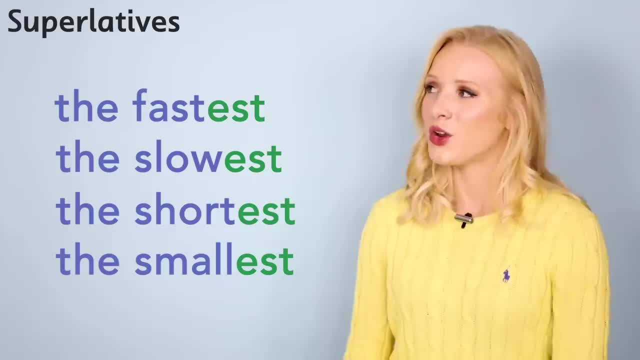 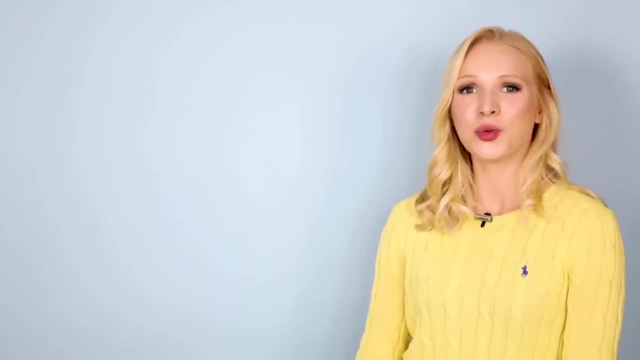 the shortest, the smallest. Notice the word the comes before the Notice the word the comes before the Notice the word the comes before the superlative. Now that you understand the differences between comparatives and superlatives. 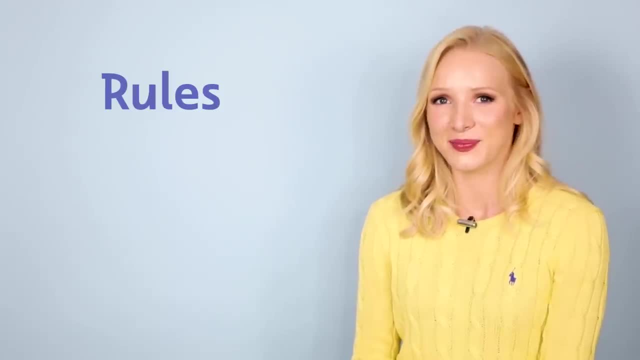 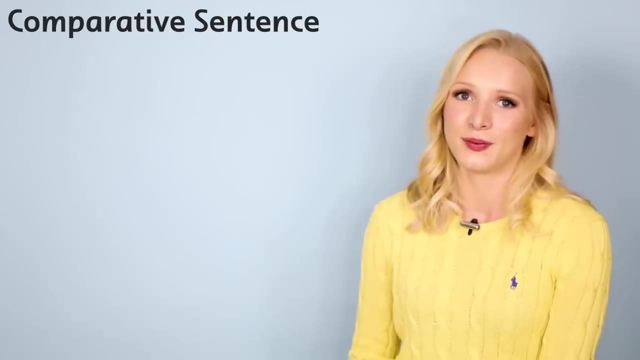 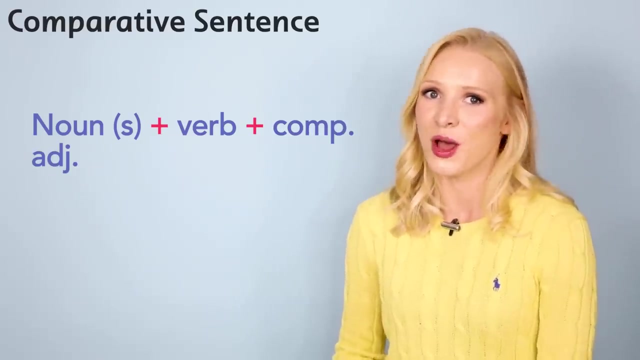 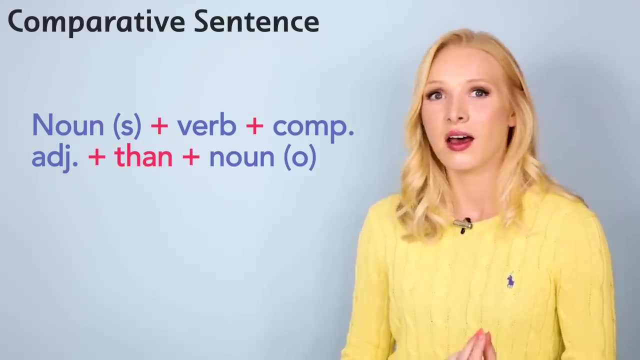 let's look at a few important rules to follow when making comparisons. Let's start by learning how to form a comparative sentence. They follow this pattern: Noun subject plus verb plus comparative adjective. plus than noun object. We must use the word than after the comparative adjective. 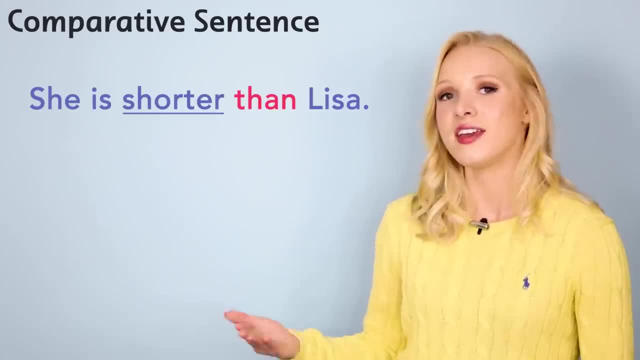 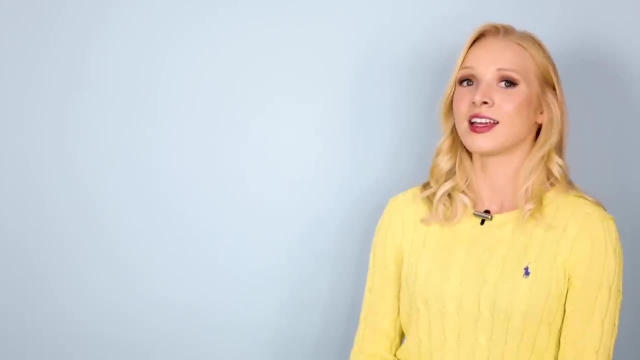 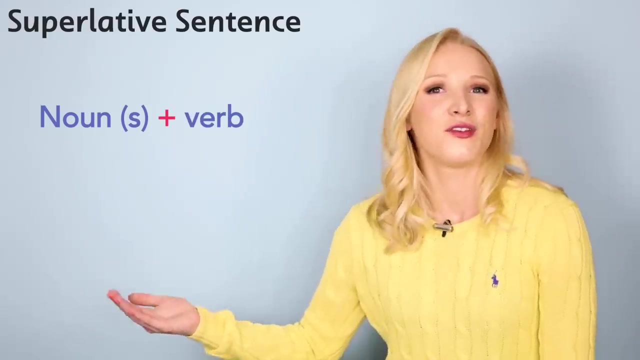 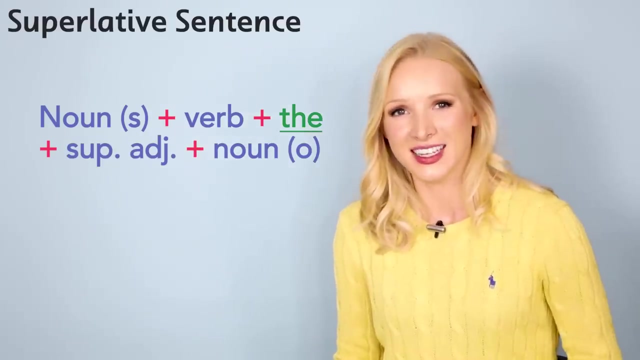 in comparative sentences. like she is shorter than Lisa, Our car is faster than his. The pattern for writing a superlative sentence is a bit different. The pattern is: subject noun plus verb plus the plus superlative adjective plus the object noun. We omit than, but place the before the superlative adjective. 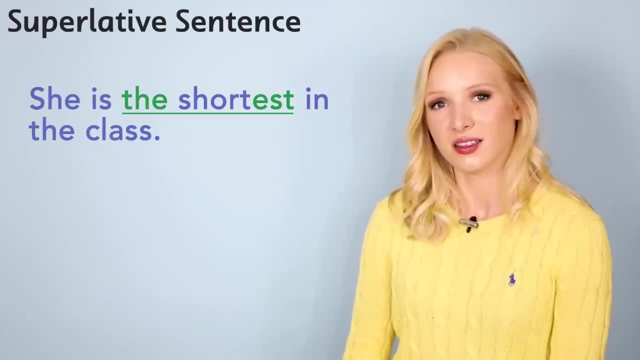 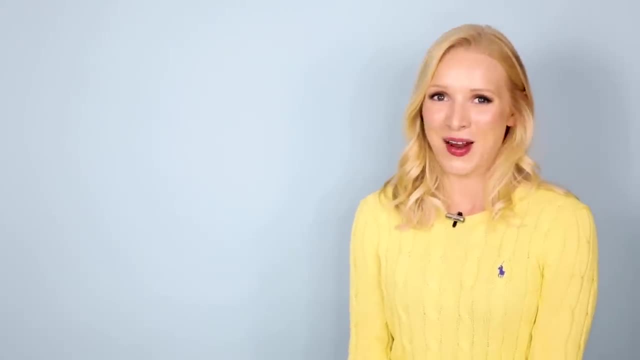 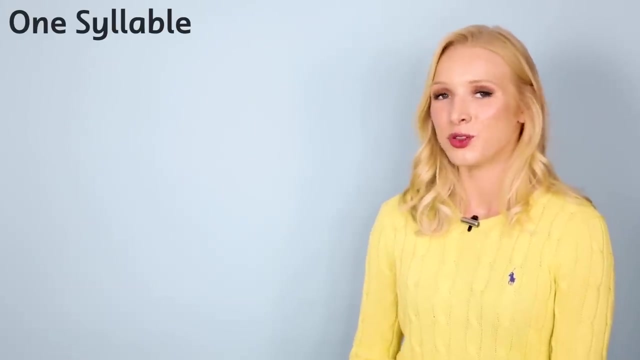 For example, she is the shortest in the class or our car is the fastest in town. Now, forming regular comparatives and superlatives is fairly easy. Let's look at a few rules For one syllable adjectives. we add er to comparatives and est to superlatives. 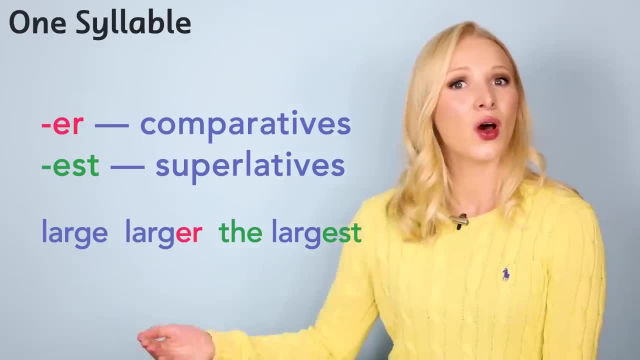 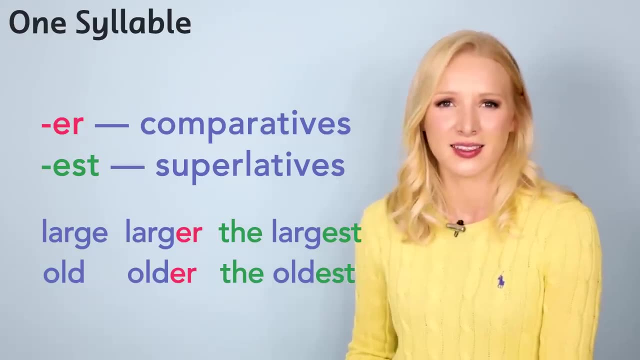 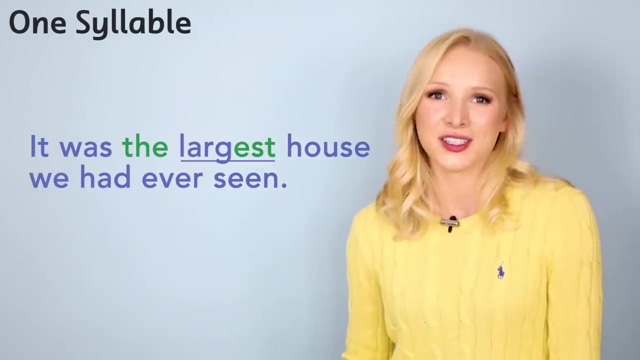 Large, larger, largest, Old, older, oldest. Notice with the superlatives, I'm not saying est oldest, I'm saying ist oldest. An example: it was the largest house we had ever seen. Adjectives that follow the consonant plus six. 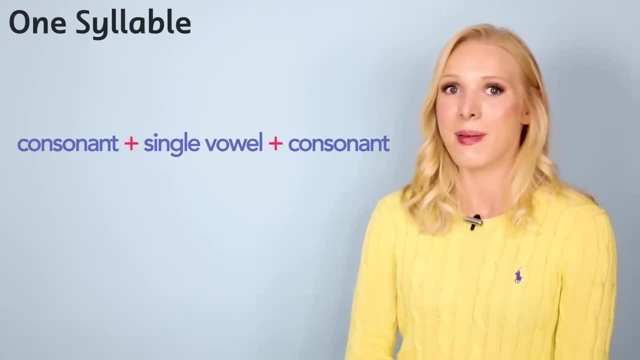 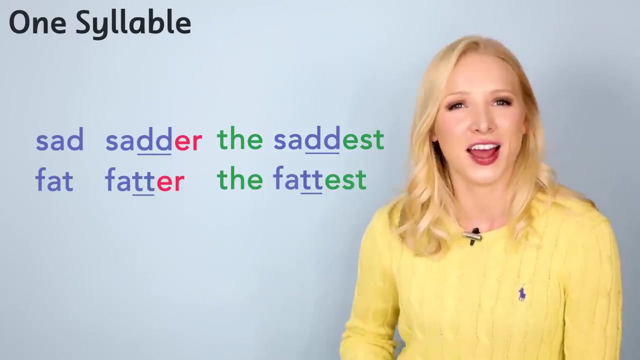 single vowel plus consonant pattern must double the final consonant. That sounds complicated, but you'll see it and it will become clear: Sad, sadder, saddest, Fat, fatter, fattest. Do you see what I mean there? 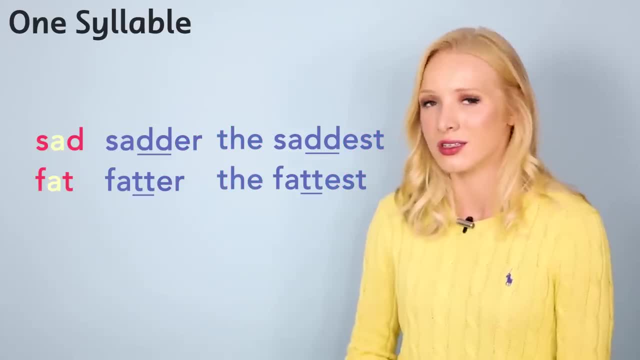 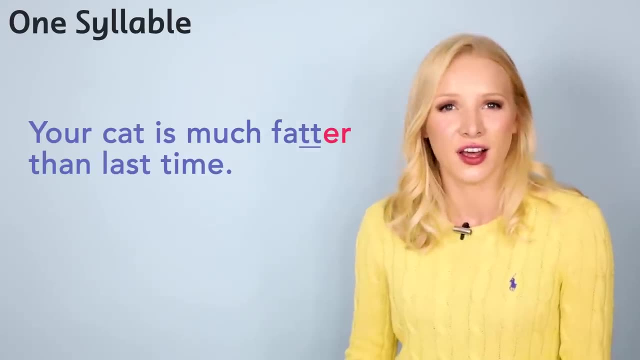 Consonant, vowel consonant. we double the final consonant to make comparatives and superlatives. An example: your cat is much fatter. Your cat is much fatter. Your cat is much fatter than last time. 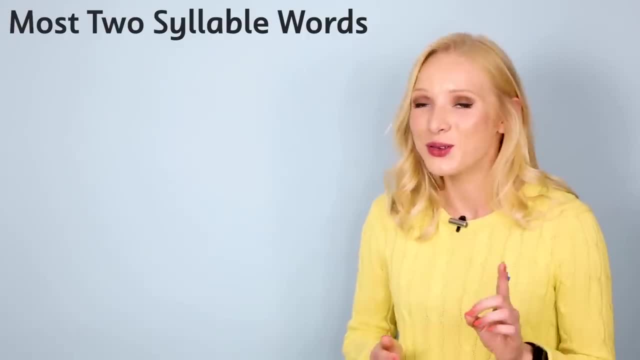 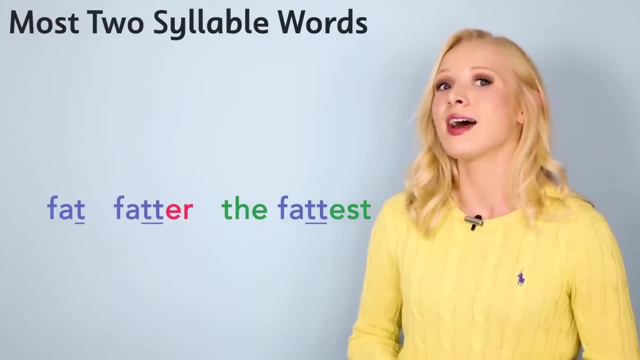 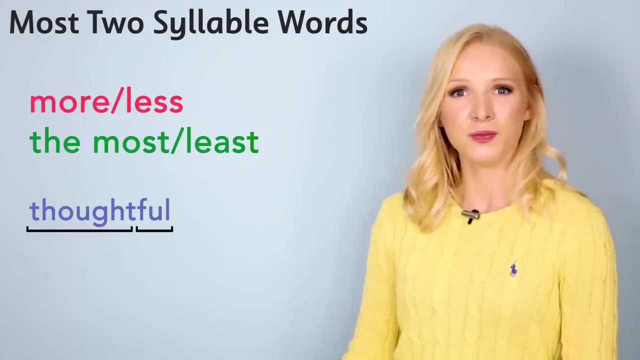 Now let's talk about most two syllable words. Not all of them- there are always exceptions- but most of them. Most two syllable comparatives will add more or less, and the superlatives will add most or least. Thoughtful, more thoughtful or less thoughtful. 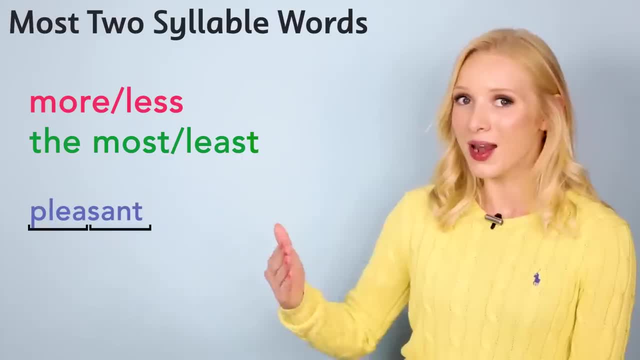 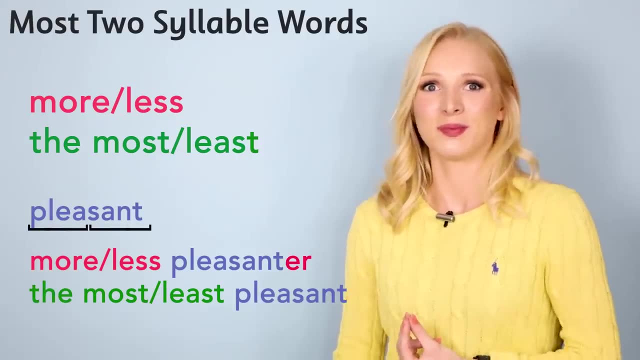 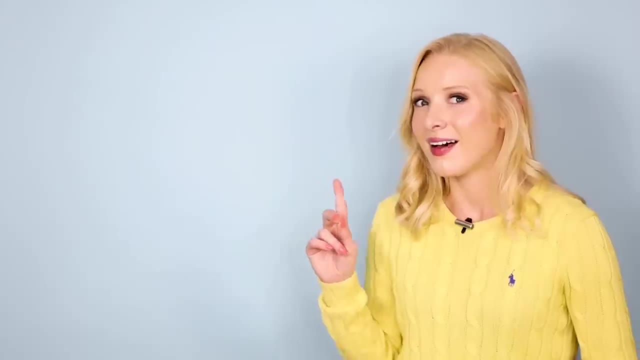 and most thoughtful or least thoughtful, Pleasant more or less pleasant, Pleasant more or less pleasant, Most or least pleasant. We don't say pleasanter or pleasantest. An example: we have the most thoughtful neighbours in this neighbourhood. There are other two syllable adjectives. 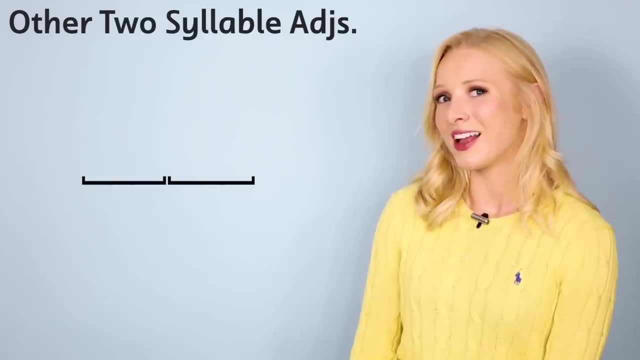 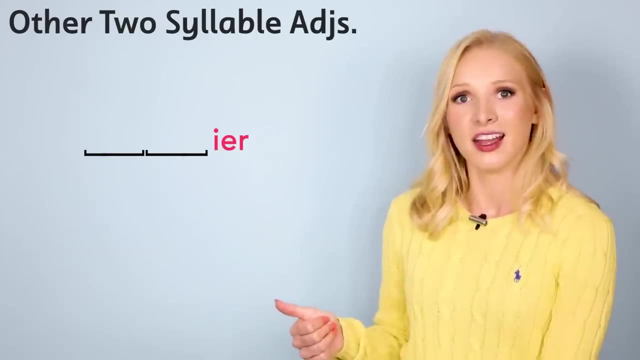 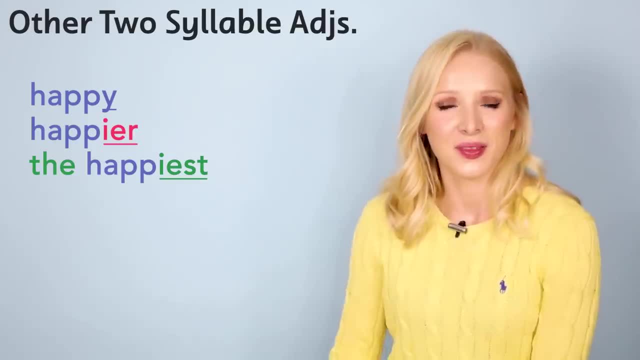 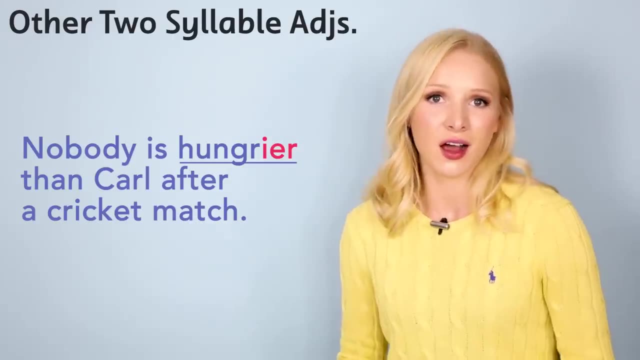 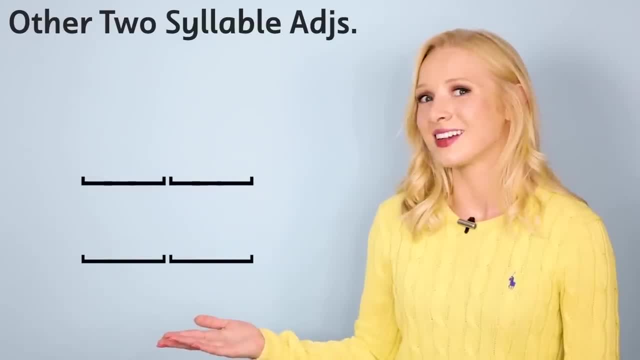 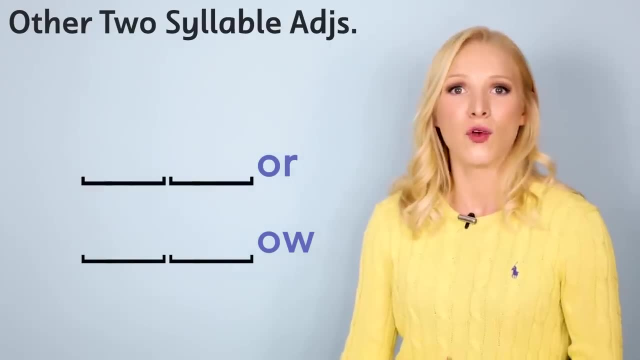 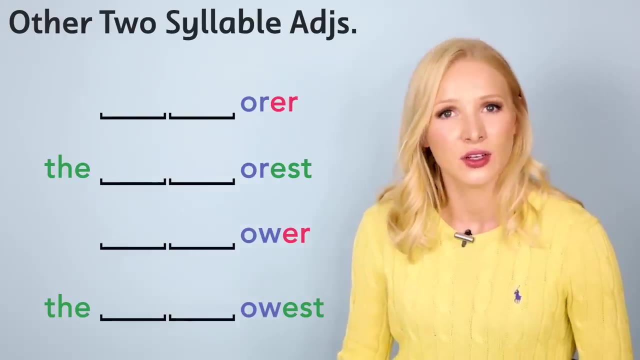 after a cricket match. We have some other two syllable adjectives. We have some ending with OR or OW which are treated like regular comparatives and superlatives. We add ER to the comparatives and EST to the superlatives. 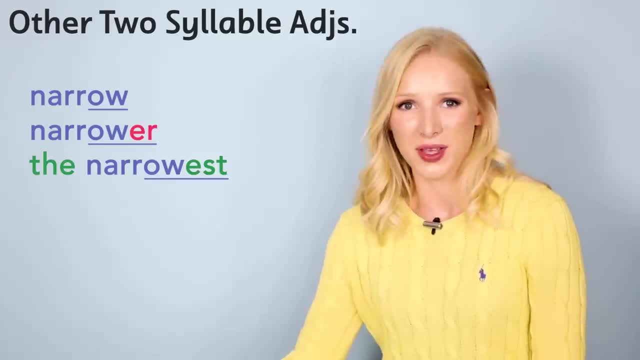 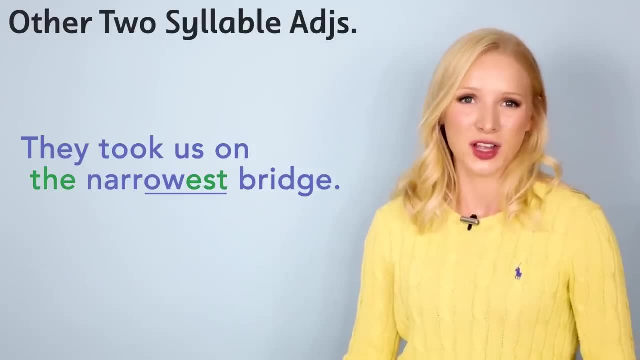 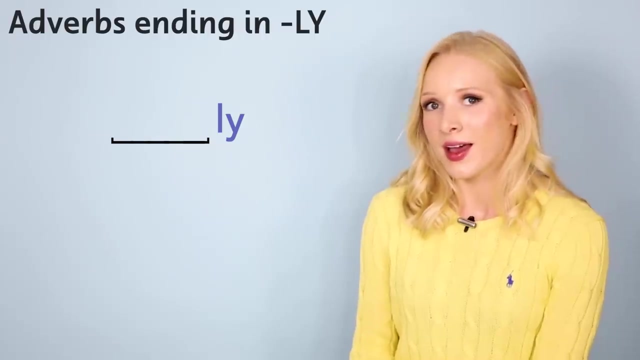 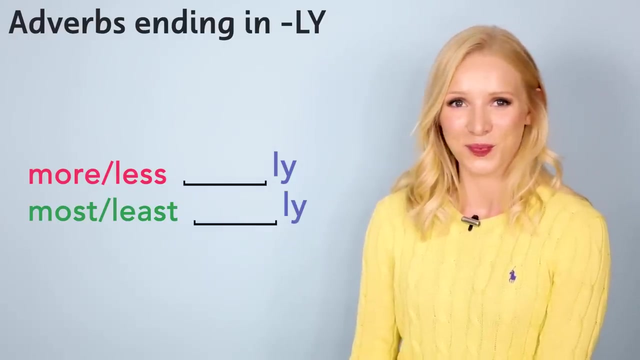 La, la, la, la la la. Narrow, narrower, narrowest, Poor, poorer, poorest. They took us on the narrowest bridge. We have adverbs ending in LY. Adverbs that end in LY receive more or less. 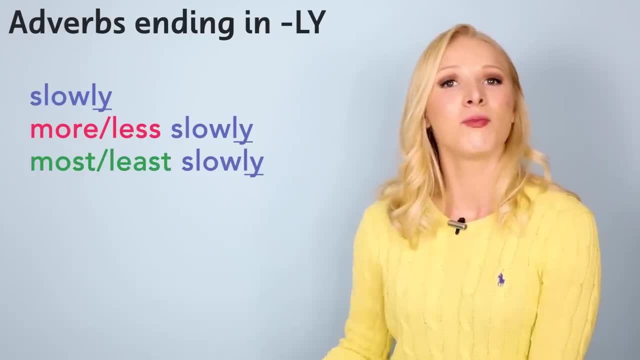 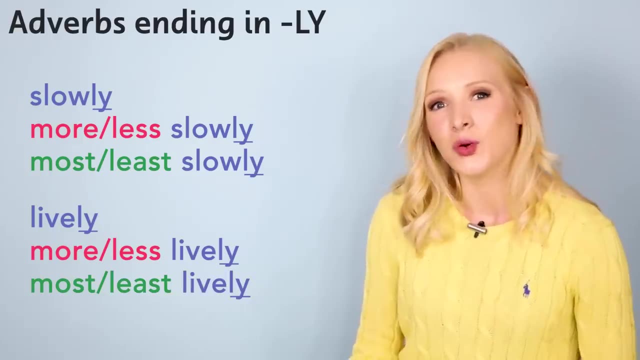 in the comparative form and, most or least, in the superlative form. Slowly, more or less slowly, most or least slowly, It becomes easier for them to say something in everyday foreign language: tonlich, Babish and crois Lively, more or less lively, most or least lively. 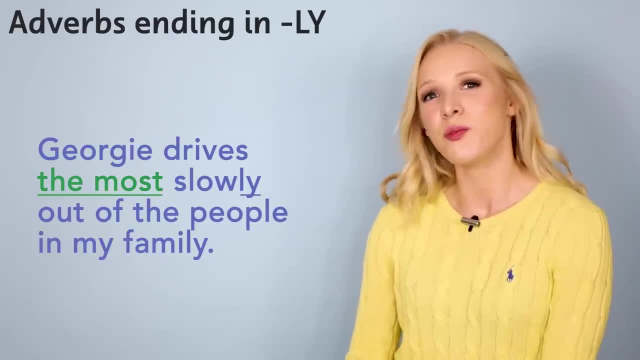 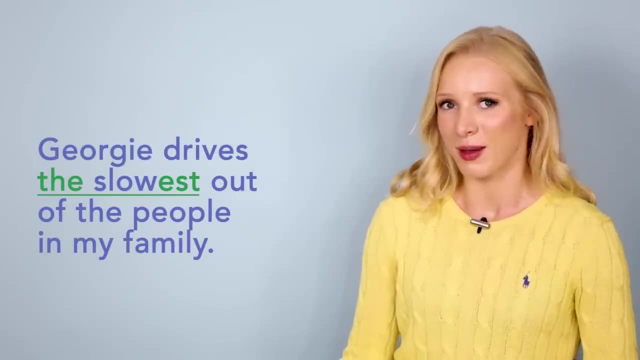 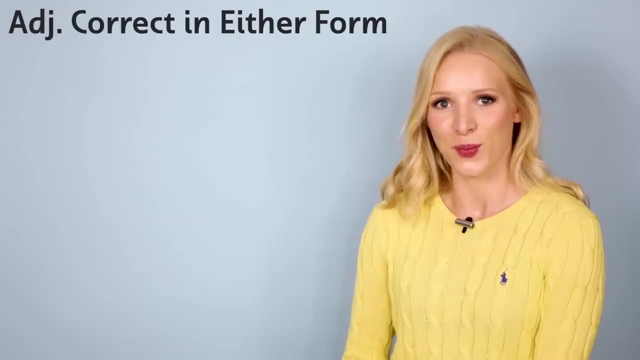 An example: Georgie drives the most slowly out of the people in my family. You could also say: Georgie drives the slowest out of the people in my family. Now this is where it gets a bit tricky. Some adjectives can be correct in either form. 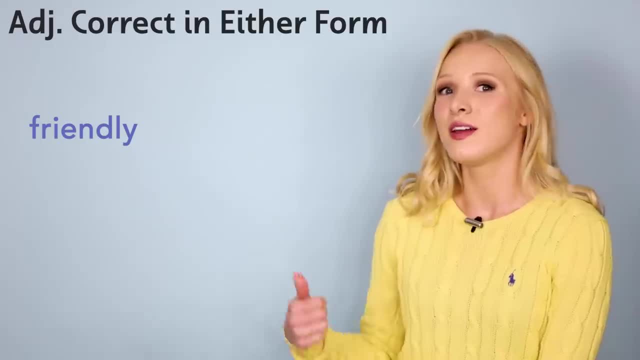 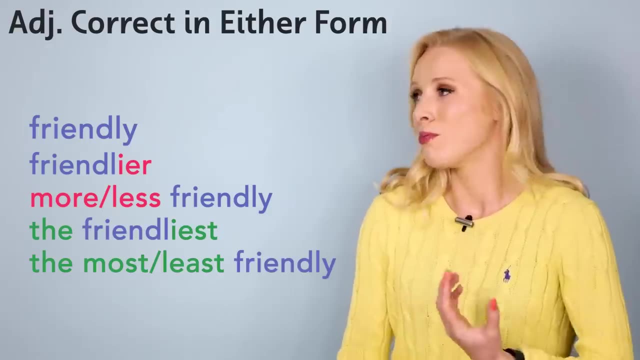 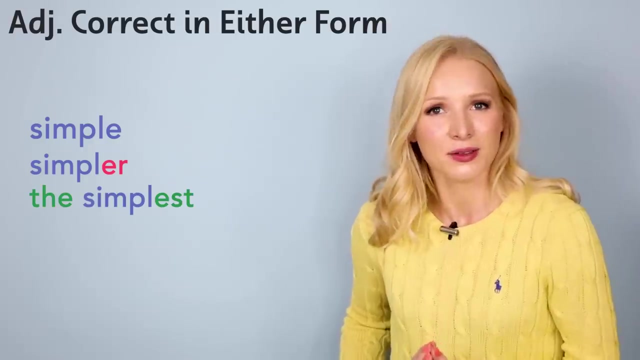 Let's look at a few examples. friendly, This can be friendlier or more. friendly or less friendly, It can be friendliest or most or least friendly. Simple is the same: simple, simpler, simplest or simple, more less simple, most least simple. 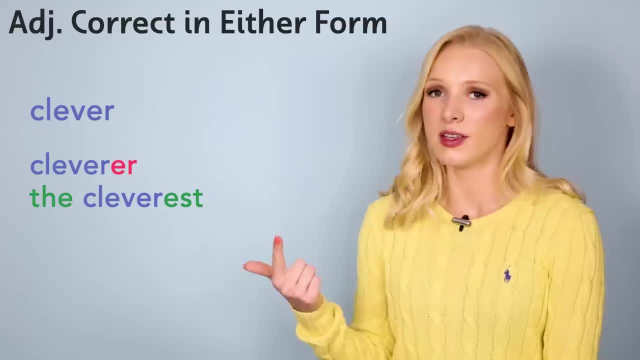 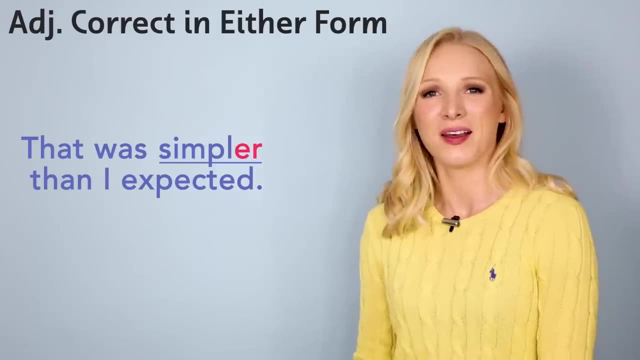 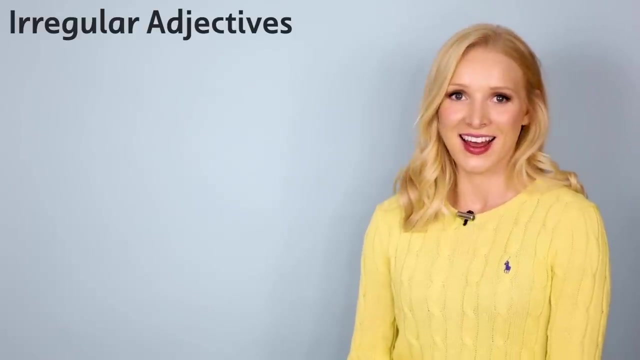 The same goes for clever- cleverer or cleverest, or more or less clever or most or least clever. An example: That was simpler than I expected Or that was more simple than I expected. There are, of course, some irregular adjectives.